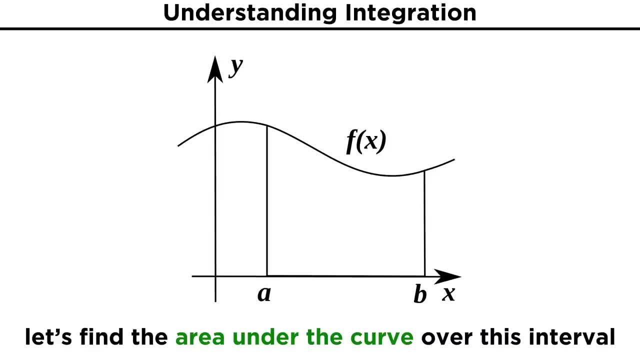 And we want to know the area under this curve, over this interval here from A to B. That means we are looking at this region S that is enclosed by the curve, the x-axis and the vertical lines. x equals A and x equals B. 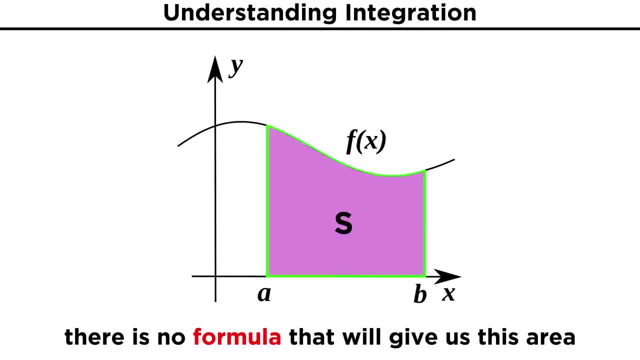 We quickly realize that there is no formula for this, as this is not a rectangle or a trapezoid or any other polygon, as polygons have only surface. So let's look at this. Let's look at this: There are so many straight line segments for sides. 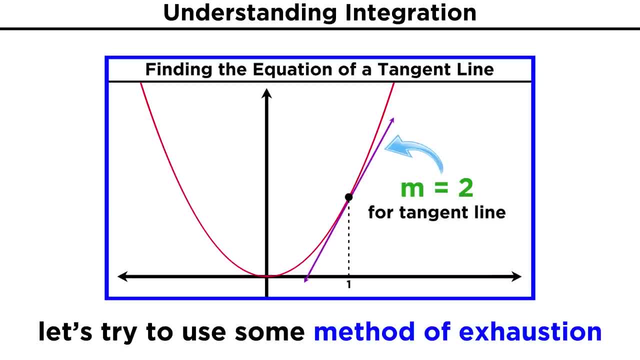 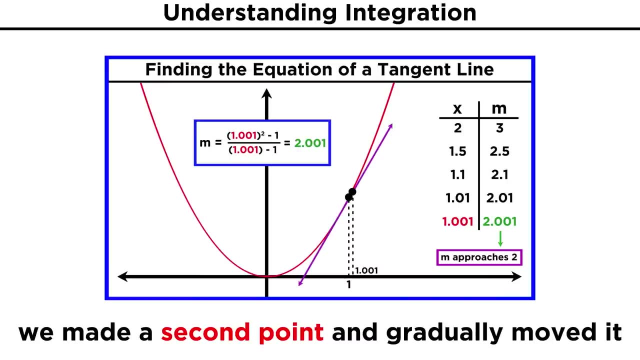 But when we first learned about differentiation, we saw that we could get the slope of a tangent line through a method of exhaustion. Can there be some parallel method here? In fact there is. When we couldn't get the slope of a line with one point, we made a second point. so 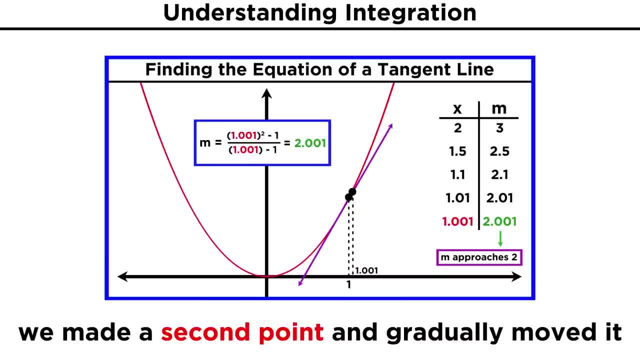 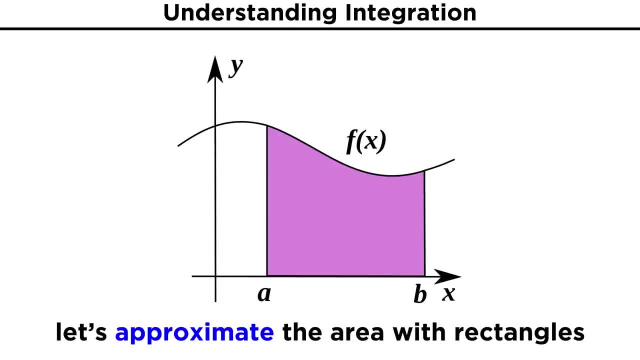 that we could get the slope and then pushed the second point towards the first point. Here we can see that the slope of the first point is the same as the slope of the second point. We can't get the area of this shape, so let's approximate it with a shape we can. 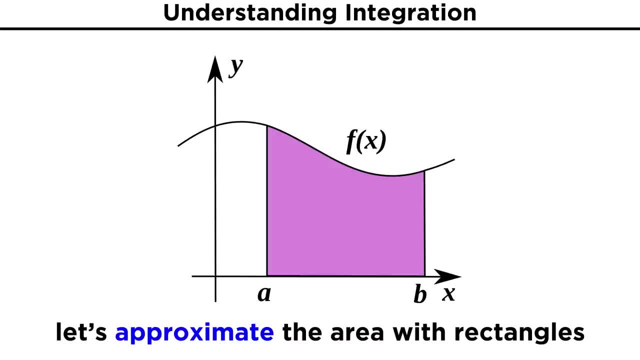 get the area of a rectangle. Let's place some rectangles and we might see that it's not the best approximation, but let's put more of them and make them narrower. That is starting to look better, as they don't stick out from the curve so much. 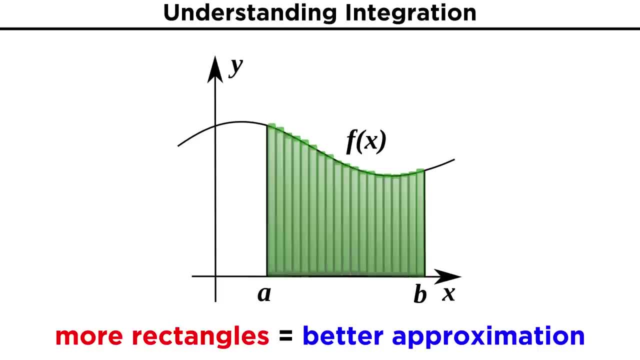 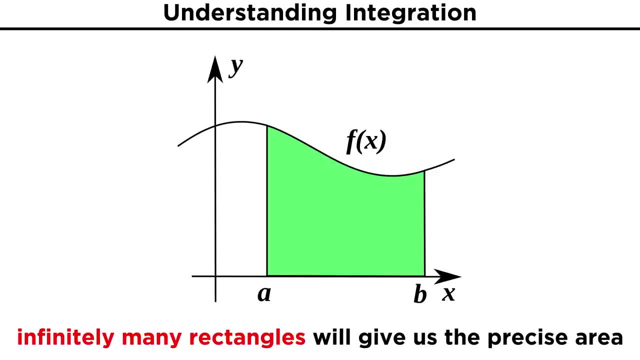 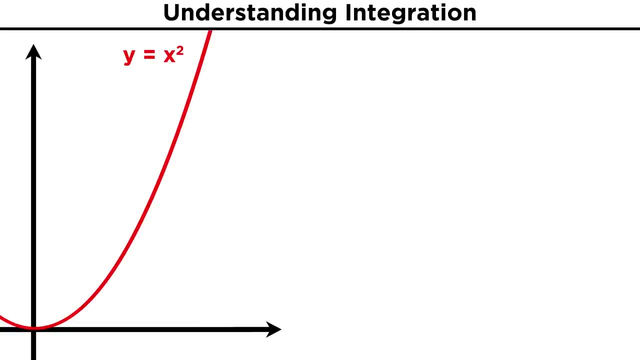 We see that as they get more and more narrow, we are more closely approximating this area. In the limit of an infinite number of infinitely thin rectangles, we will get the precise area under this curve. Let's do this more quantitatively on a specific function to get a better grasp of what's. 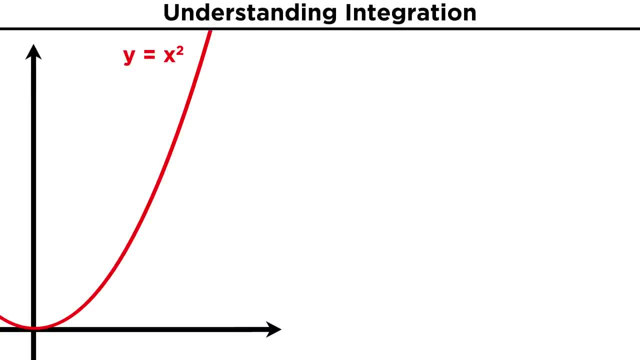 going on. Let's take Y equals X. squared, Say we want to know the area under this curve over the interval of zero to one. so let's write in the point and label this shaded region S. We know that this area must be somewhere in between zero and one because a square 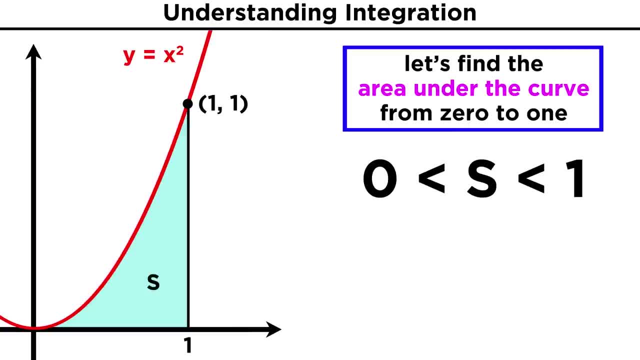 with these sides will have an area of one, and this area is smaller than that. But let's use some rectangles and see how close we can get. First, let's chop this area up into four sections, from zero to one. fourth, then to: 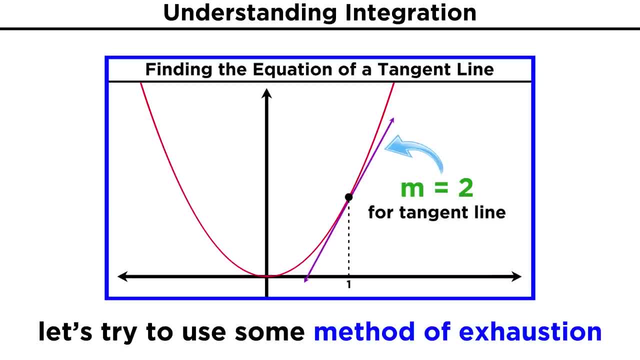 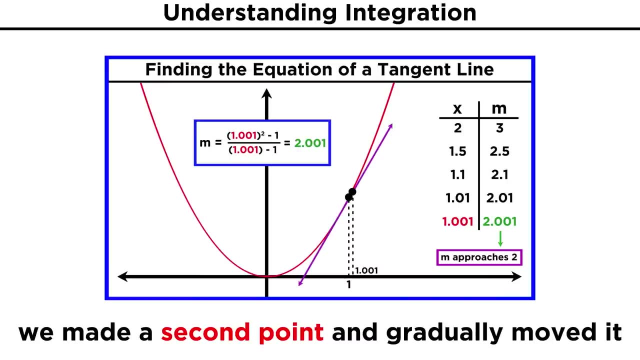 But when we first learned about differentiation, we saw that we could get the slope of a tangent line through a method of exhaustion. Can there be some parallel method here? In fact there is. When we couldn't get the slope of a line with one point, we made a second point. so 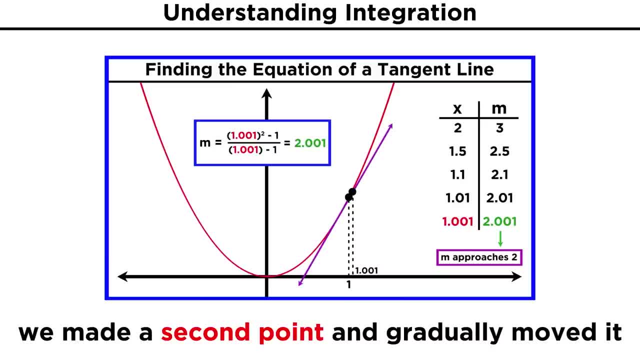 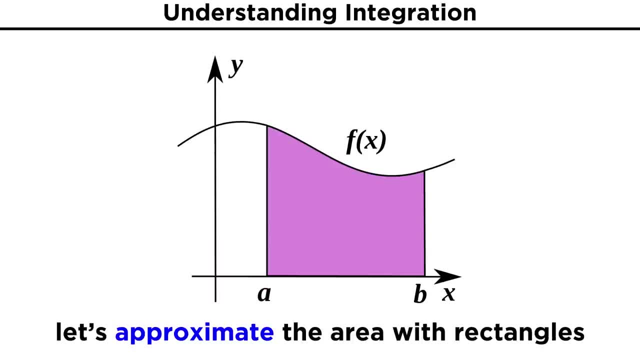 that we could get the slope and then pushed the second point towards the first point. Here we can see that the slope of a tangent line is equal to the slope of a tangent line. We can't get the area of this shape, so let's approximate it with a shape we can. 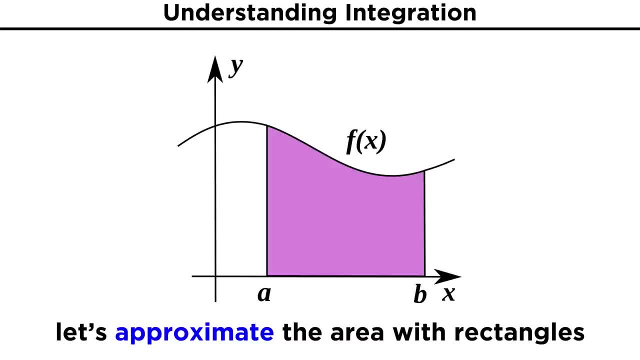 get the area of a rectangle. Let's place some rectangles and we might see that it's not the best approximation, But let's put more of them and make them narrower. That is starting to look better, as they don't stick out from the curve so much. 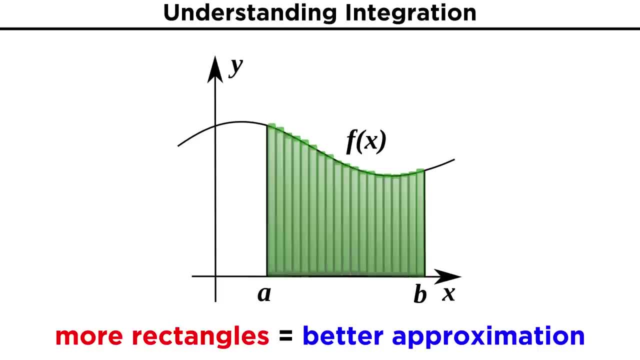 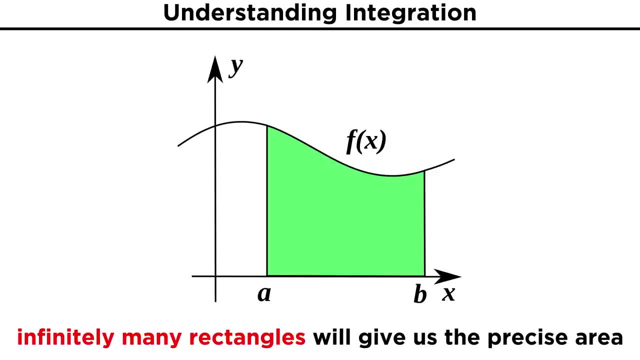 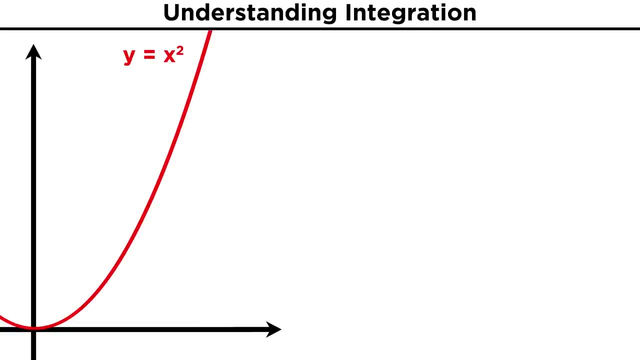 We see that as they get more and more narrow, we are more closely approximating this area. In the limit of an infinite number of infinitely thin rectangles, we will get the precise area under this curve. Let's do this more quantitatively on a specific function to get a better grasp of what's. 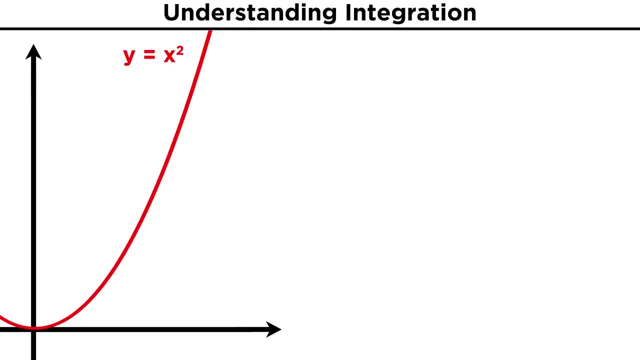 going on. Let's take Y equals X. squared, Say. we want to know the area under this curve over the interval of zero to one. so let's read in the point and label this shaded region S. We know that this area must be somewhere in between zero and one, because a square with 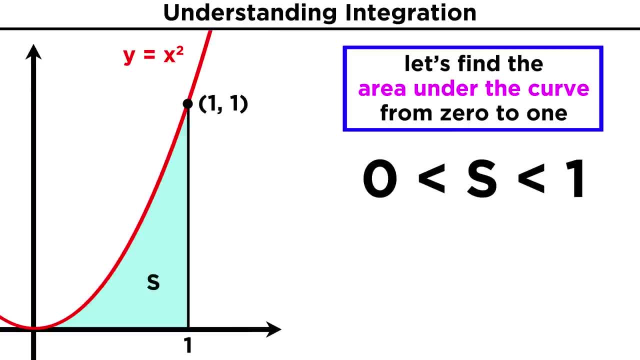 these sides will have an area of one, and this area is smaller than that, But let's use some rectangles and see how close we can get. First, let's chop this area up into four sections, from zero to one-fourth, then to 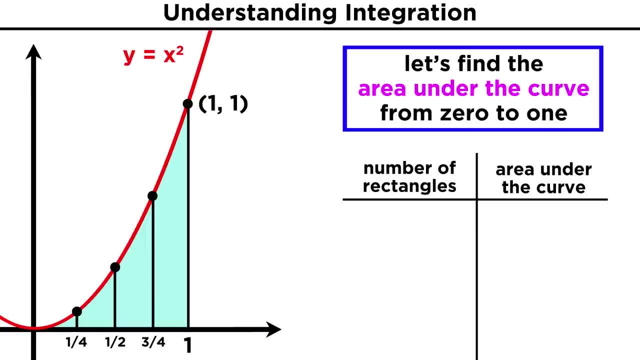 one-half, then to three-fourths, then to one-third, Then to one. We can approximate each of these with a rectangle, which is useful because it will be easy to get the areas of these rectangles. Each of them has a base of one-fourth and we can get the heights by using the function. 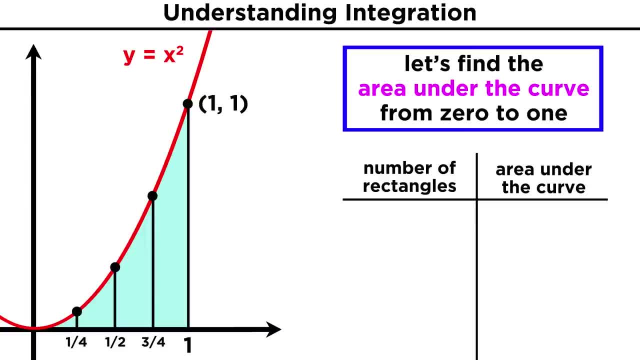 one, half, then to three, fourths, then to one. We can approximate each of these with a shape. Let's do this more quantitatively. on a specific function. so let's write in the point and label this area under this curve, over the interval of zero to one. so let's write in: 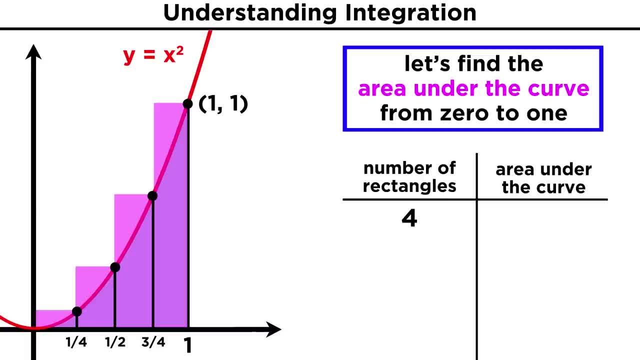 the point and label this area up into four sections, from zero to one fourth, then to one half, then to one half. We can approximate each of these with a rectangle, which is useful because it will be easy to get the areas of these rectangles. 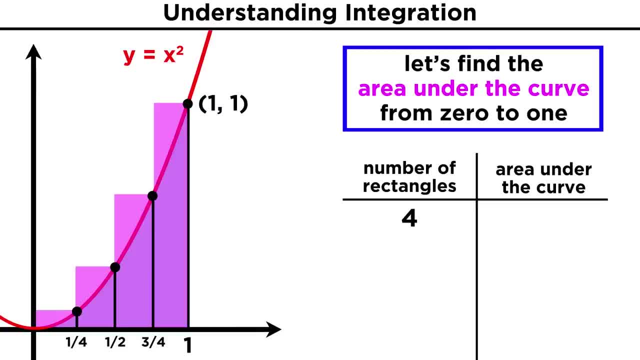 Each of them has a base of one fourth and we can get the heights by using the function. The X coordinate of this point is one fourth and every point on this curve has the coordinates X- X squared. so the height of this first rectangle must be one fourth squared, or one. 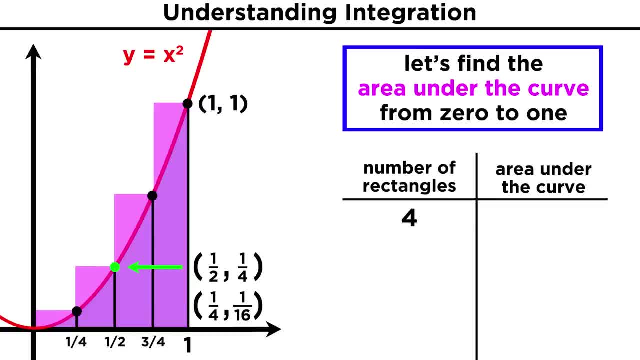 sixteenth. The second rectangle has a height of one half squared, or one fourth. The third rectangle has a height of nine sixteenths and the fourth has a height of one. We know that the area of a rectangle is base times height, so we just multiply these values. 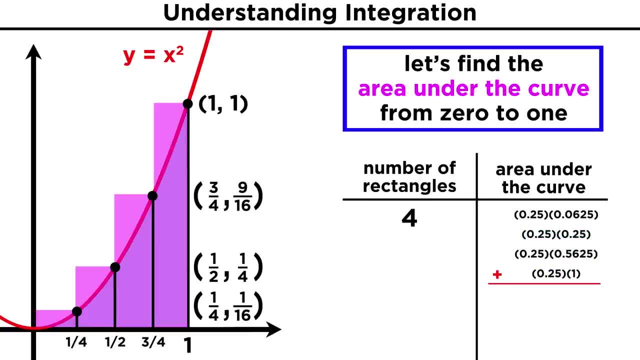 together to get the area of each rectangle and add them up to get the total area. This is around zero point four six nine. So this is our first rough approximation. We know that the true value is less than this because these rectangles stick out above the 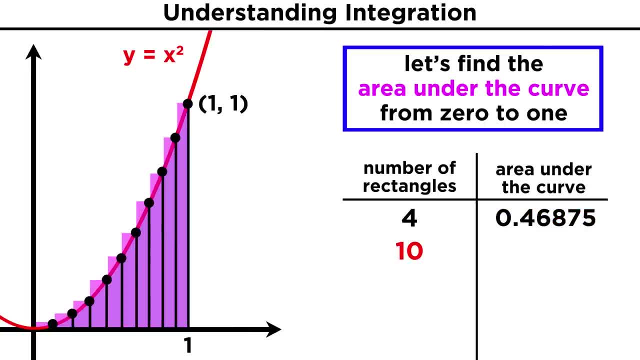 curve. But now let's use ten rectangles and see what that gives us. These rectangles will all have a base of one tenth, as well as the following heights and therefore these corresponding areas. Again, we simply add up the areas and we get zero point three, eight, five. 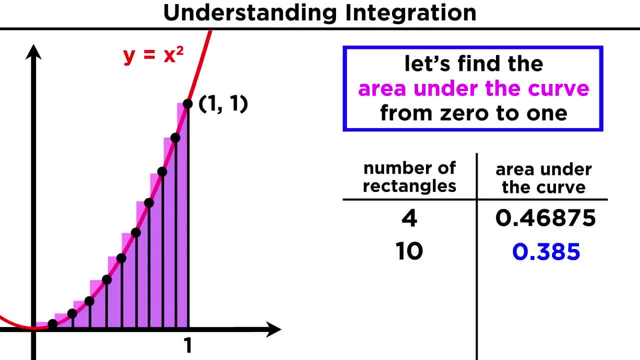 This looks like it is much closer to the area we are looking for because the rectangles don't stick out past the curve as much as before. We can use smaller and smaller rectangles to get closer and closer to the precise area, and while we won't show hundreds of rectangles here, this table illustrates what happens. 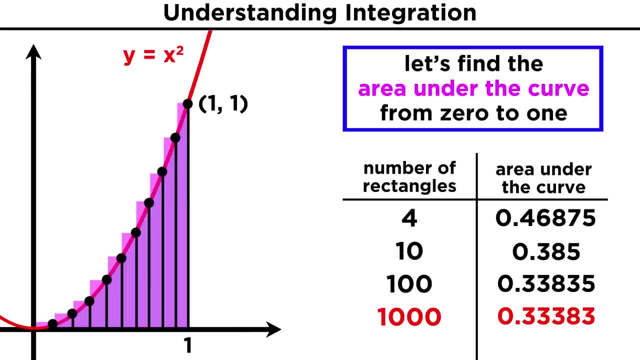 as the number of rectangles increases. If we go back to our first rectangle, we can see that after we take the same number of rectangles, the number of rectangles gets larger, all the way up to a thousand. We can clearly see that this area is getting closer and closer to a specific value and 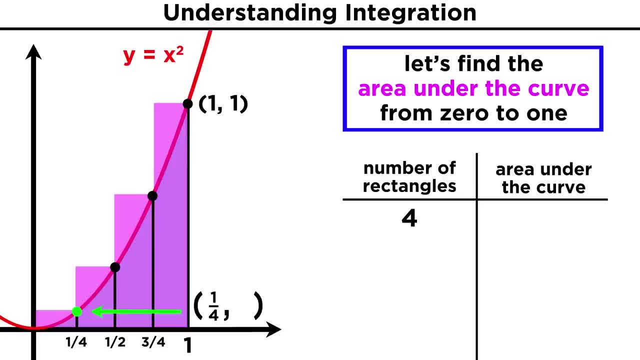 The X coordinate of this point is one-fourth and every point on this curve has the coordinates X, X squared. so the height of this first rectangle must be one-fourth squared, Okay, Or one-sixteenth. The second rectangle has a height of one-half squared, or one-fourth. 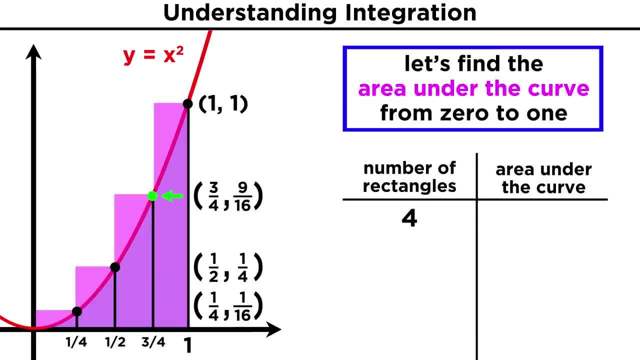 The third rectangle has a height of nine-sixteenths and the fourth has a height of one. We know that the area of a rectangle is base times height, so we just multiply these values together to get the area of each rectangle and add them up to get the total area. 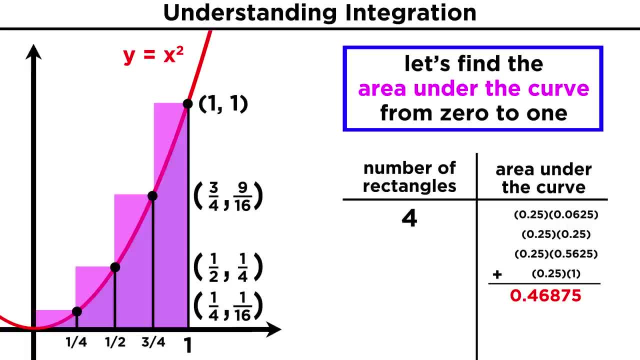 This is around zero to one-fourth. Zero point four six nine. So this is our first rough approximation. We know that the true value is less than this because these rectangles stick out above the curve. But now let's use ten rectangles and see what that gives us. 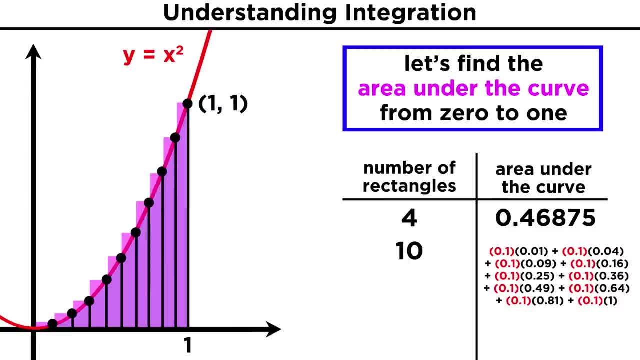 These rectangles will all have a base of one-tenth, as well as the following heights And therefore these corresponding areas. Again, we simply add up the areas and we get zero point three, eight, five. This looks like it is much closer to the area we are looking for, because the rectangles 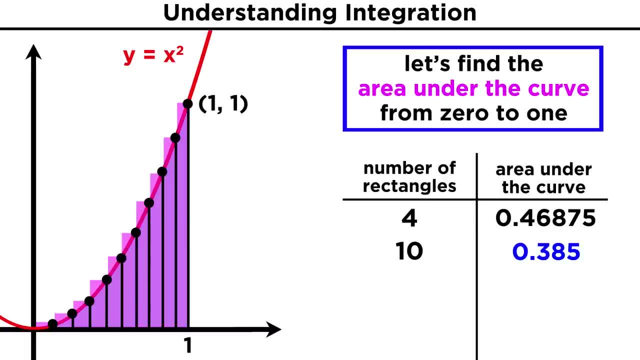 don't stick out past the curve as much as before. We can use smaller and smaller rectangles to get closer and closer to the precise area, and while we won't show hundreds of rectangles here, This table illustrates what happens as the number of rectangles gets larger, all the 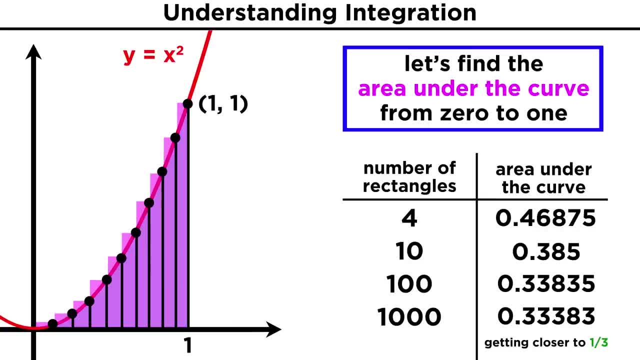 way up to a thousand, We can clearly see that this area is getting closer and closer to a specific value, and that value is one-third. In the limit of an infinite number of rectangles, the sum of the areas of the rectangles will be precisely one-third. therefore, the area under this curve is equal to one-third. 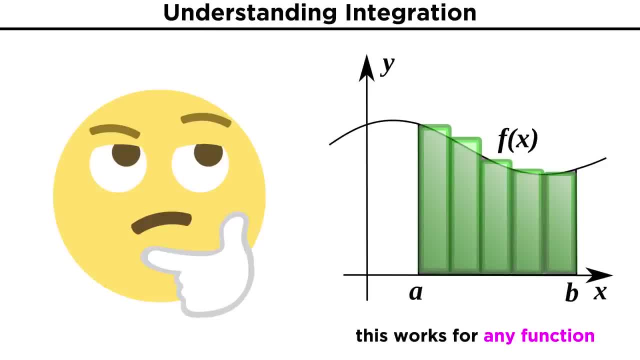 We can apply this generally to any function, like the first one we looked at. However many rectangles we use, we can represent the sum of their areas using summation notation which, as we recall from an earlier tutorial, involves this uppercase sigma which just